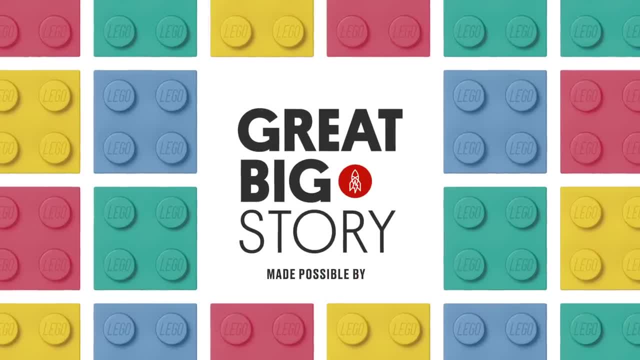 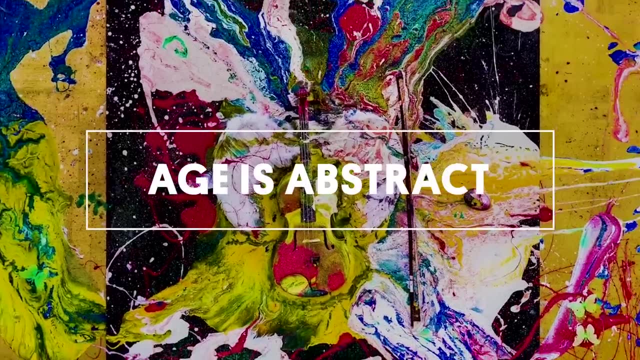 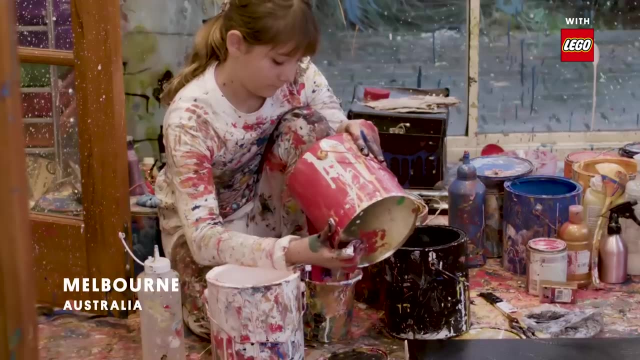 else. This great big story was made possible by Lego. Play her way. My name is Alita Andre. I'm an abstract painter and I'm from Melbourne, Australia. At only 12 years old, Alita has been in the industry for over a decade. 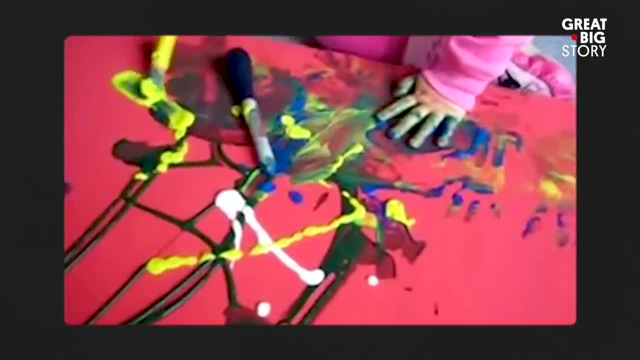 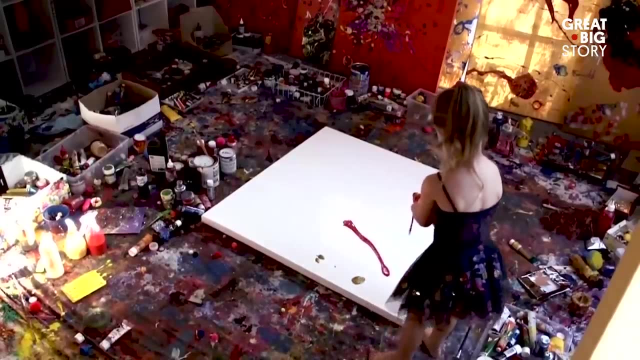 I started painting. when I was nine months old, My dad put a canvas down on the floor because he used to paint a little bit. I just started crawling on the canvas and started painting before him. That's how it all started. That's how it all started. 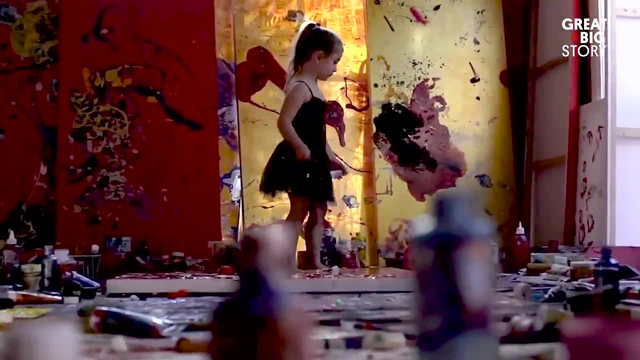 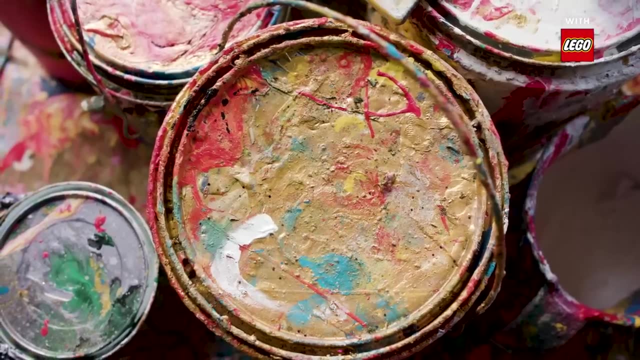 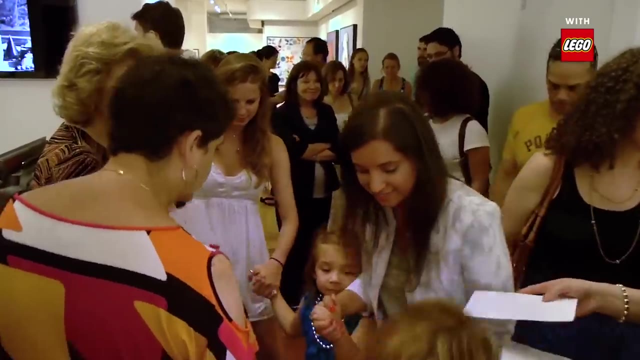 That was my first painting. Well, my first show was at the age of two years old. Without telling the gallery owner her age, her mother presented the work and Alita was booked for her first show. Since then, she has taken her art across the globe and has 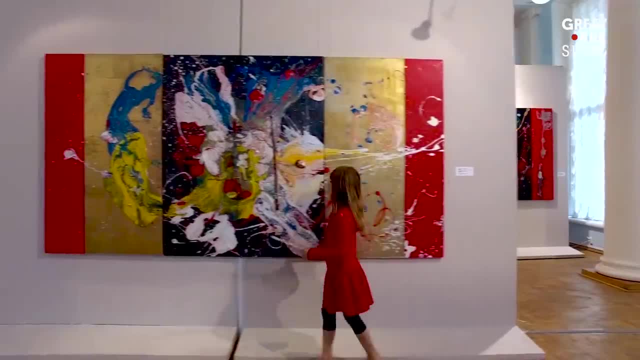 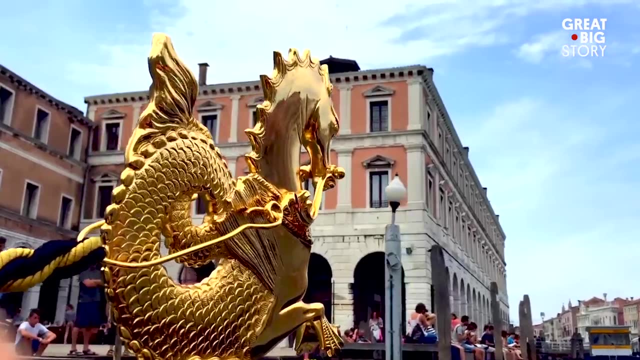 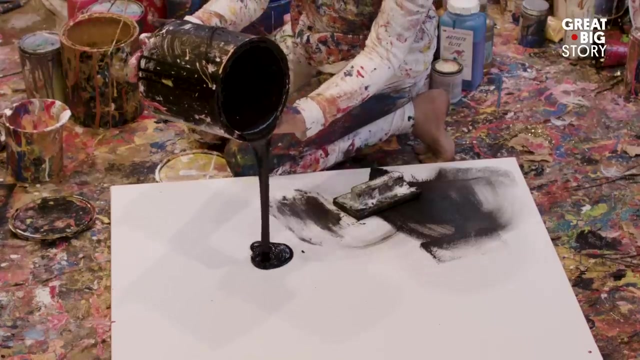 sold paintings for around US$35,000.. I've been to London, Russia, Japan, New York, Italy, China, Montmorency, Hong Kong, but four times. I paint every few days, but mainly when I'm inspired. When I paint, I usually think about. 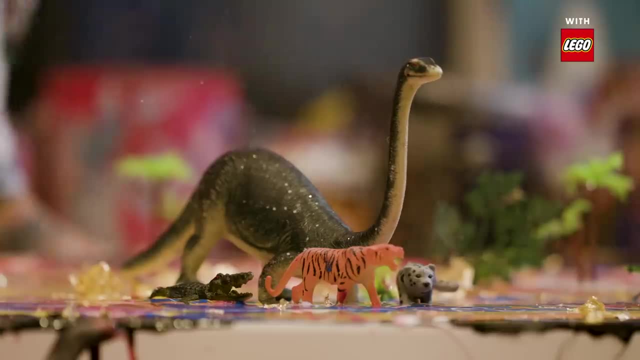 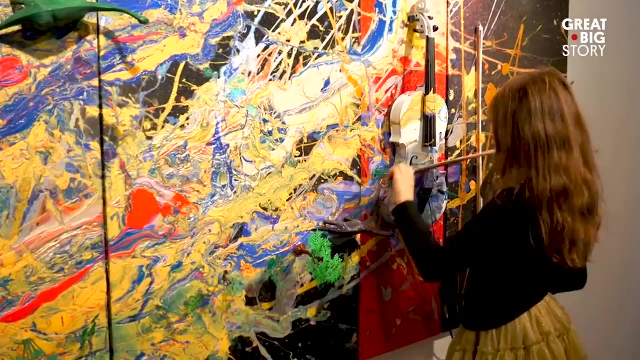 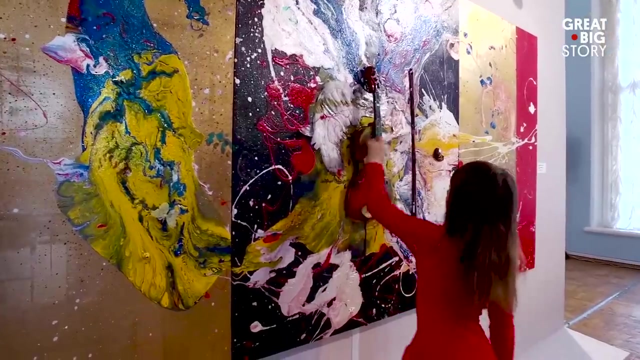 the universe. I think about animals, pretty much everything that has to do with nature, With the violins on the canvas. I want to show that the whole universe is singing. I'm going to show that the whole universe is singing. Although Alita's young, she understands the harsh critics in the art world. 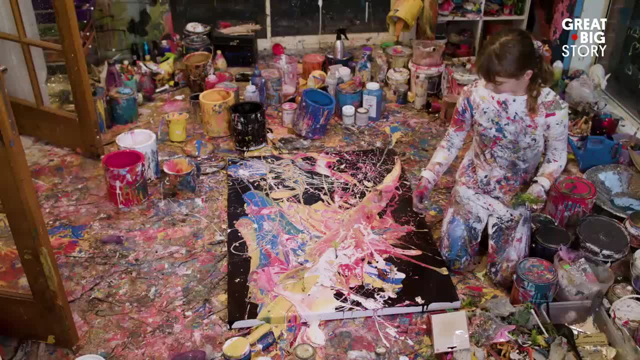 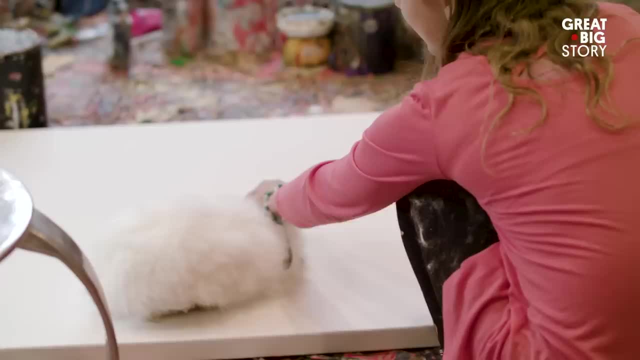 When people question my talent, usually I don't mind, because I think that everyone should have their own opinion. But there is one critic whose opinion does matter. So Fluffy is our little pet art critic. He usually starts biting me or biting the painting. 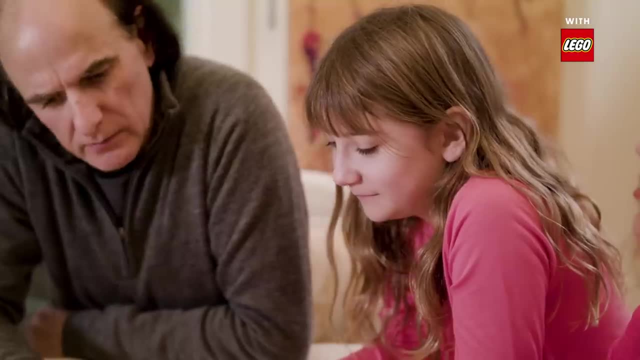 if he doesn't like it. My mum and dad encouraged my art and I'm so happy. So Fluffy is our little pet art critic. He usually starts biting me or biting the painting if he doesn't like it. My mum and dad encouraged my art and I'm so happy. So Fluffy is our little pet art critic. He usually starts biting me or biting the painting if he doesn't like it. So Fluffy is our little pet art critic. He usually starts biting me or biting the painting if he doesn't like it. 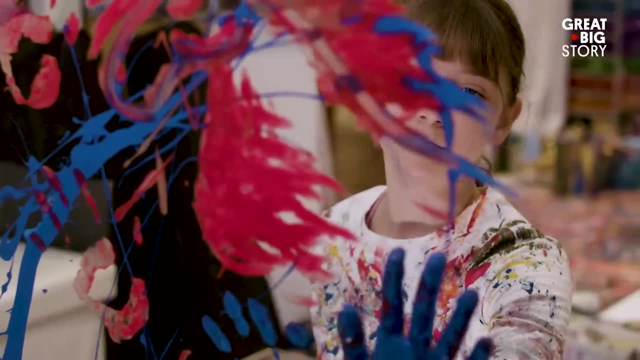 So I definitely think that I'm going to be doing painting for the rest of my life. It's something that I love so much.